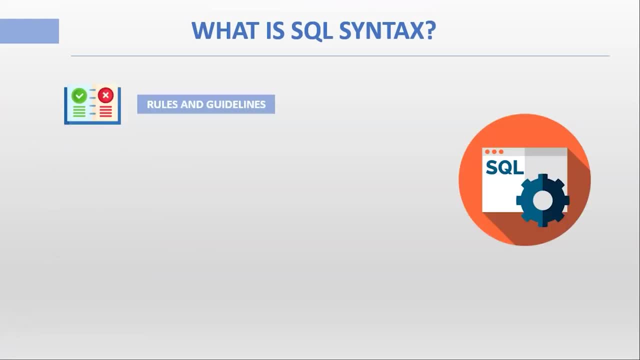 What is SQL Syntax? Just like other programming languages, SQL follows a unique set of rules and guidelines called Syntax. We use simple English words in the SQL Syntax in order to create various queries. SQL Syntax is, by default, case-insensitive. That means the system allows the user to write. 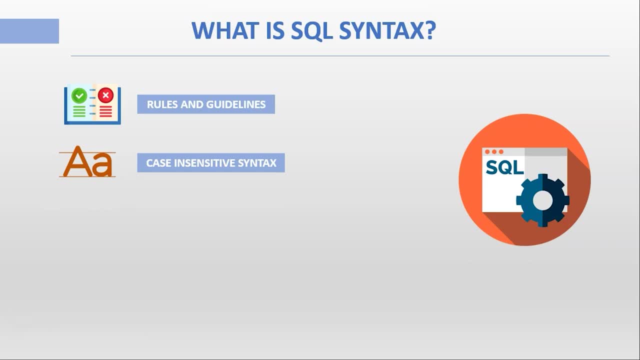 the queries in both uppercase as well as lowercase, But if you're working with MySQL Server, then you need to give table names exactly as they exist in the database. We know that RDBMS is the basis for all modern database systems, including SQL, which manages 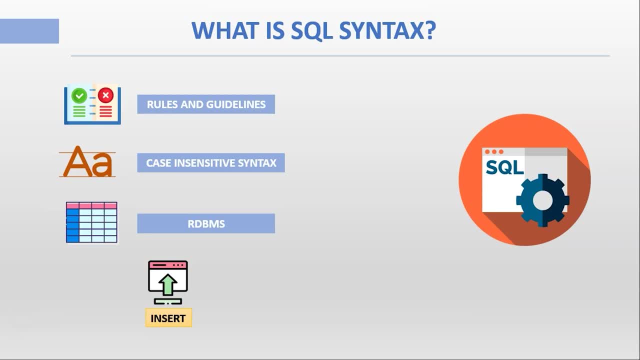 and performs various operations on the tables, like Insert, Update, Modify and Delete. So in order to retrieve the data stored in the database, it is necessary to learn SQL Syntax first Before we move ahead with the topic. if you want to learn more about the basics of DBMS, 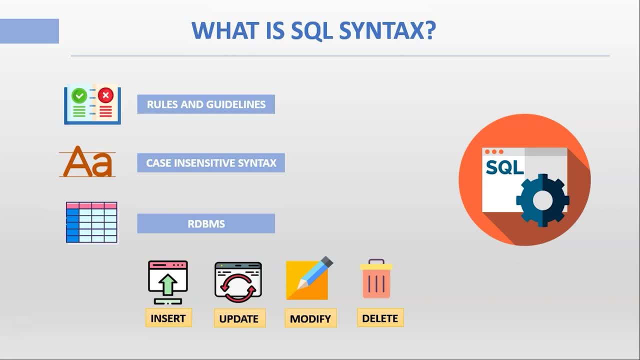 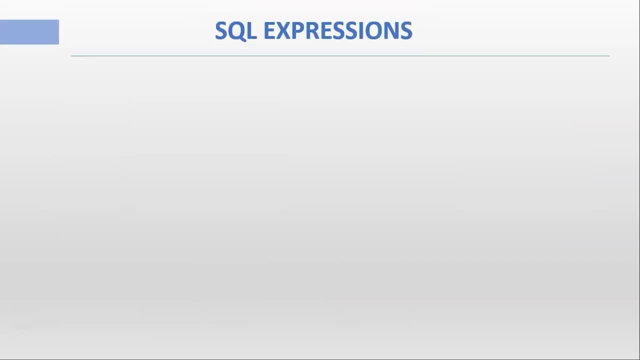 and SQL. make sure you check out our previous playlist videos on Introduction to DBMS and SQL on our channel. We'll leave the link in the description below. SQL Expressions. SQL Expressions is a combination of one or more keywords and values: operators. 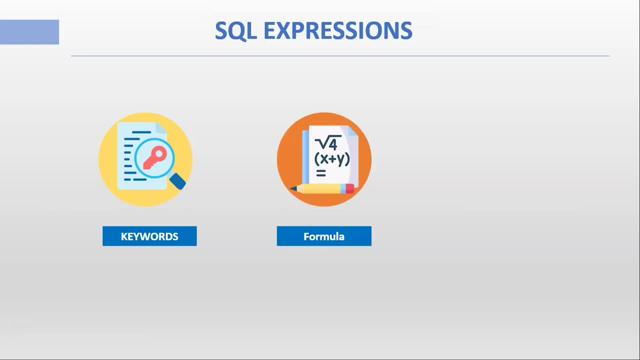 data types and other SQL functions. These SQL Expressions are like a formula, which are similar to mathematical formulas which we generally use to solve a problem, And in this case they're written in a query language using a proper syntax. SQL Statement- SQL Statements are basically a collection of SQL Expressions. For example: 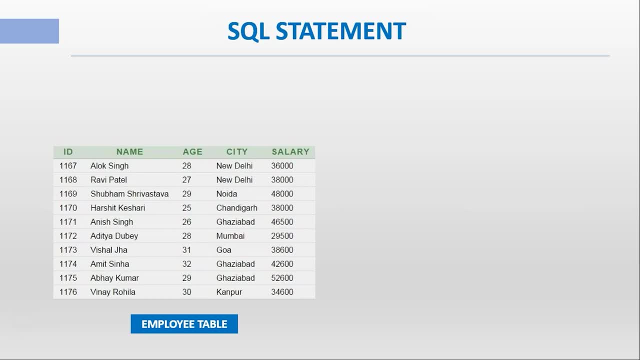 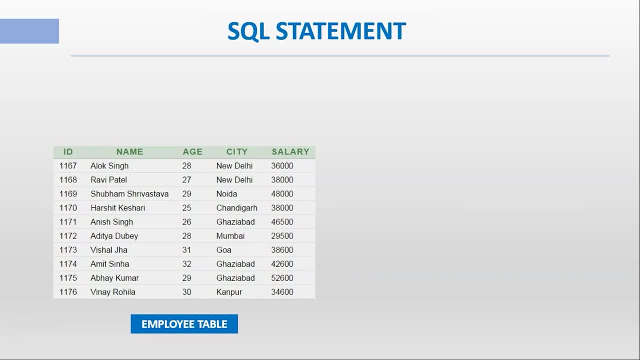 Age, City and Salary. Now, if I want to fetch the record of all the employees and their IDs, I'll write a simple SQL query That is SELECT ID NAME FROM EMPLOYEE. Here SELECT is the database object or the keyword that is used, ID and NAME are the columns. 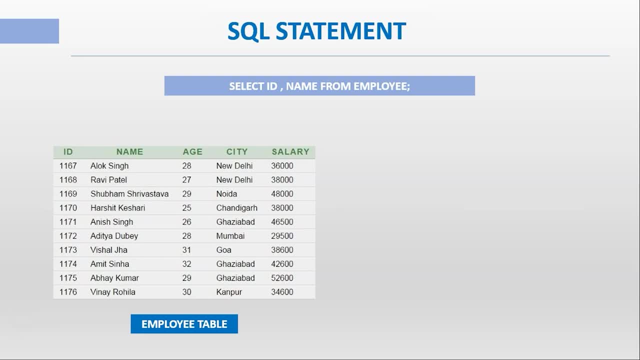 from EMPLOYEE. EMPLOYEE is the name of the table. When I execute this query, this will be the output. It will display the ID and name of the employee. Let us look at another query Now. I want to display the salary of employees having 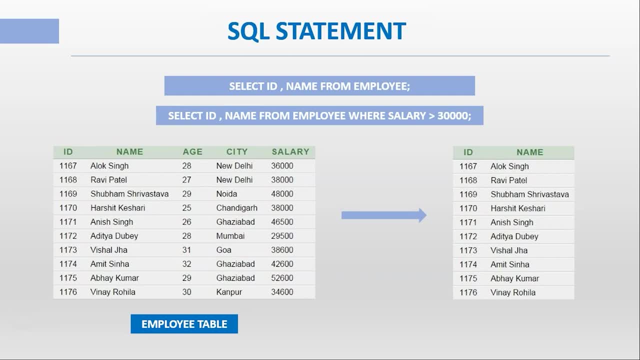 more than 30,000.. For that, I am using the query as SELECT ID NAME FROM EMPLOYEE WHERE SALARY is greater than 30,000.. Here, WHERE is the conditional statement that I am using, or it is a SQL clause? Also, we are using greater than symbol, which is an SQL operator. 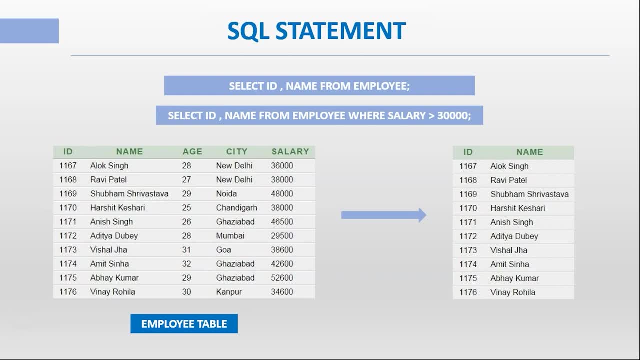 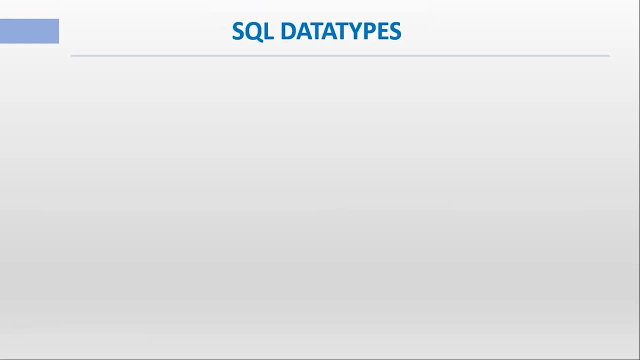 So, with the help of SQL statements, we can fetch the records of all the information from SQL tables. SQL data types. SQL data types specifies which type of values is stored in the database tables. SQL data types are mainly classified into three categories. The first one is Numeric. 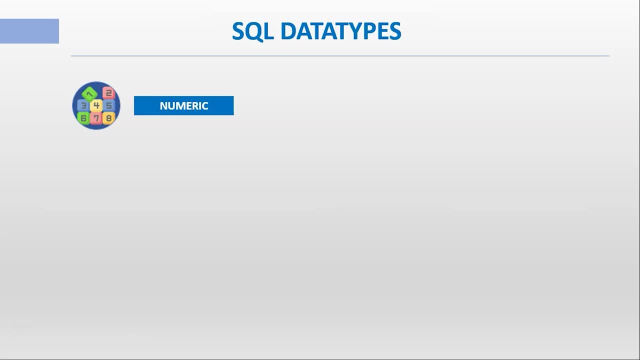 Numerical data refers to the data that is in the form of numbers. In numerical data type we have different types as well, For example INT. INT holds values of integers and whole numbers without any decimal point. Further, they are again divided into small int and big int. also, The difference between 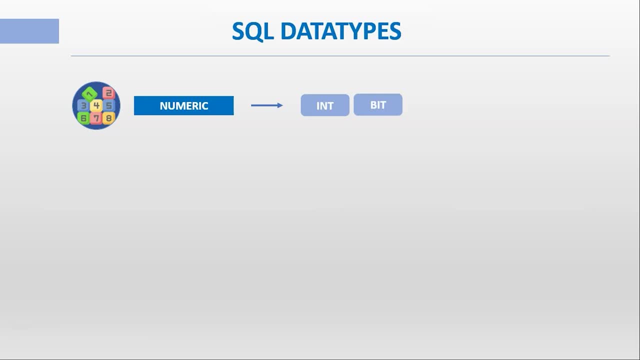 them is the size and range of the value they can store and operate Bit. Bit data type is an integer data type that can only take values of 0,, 1 or any null value. SQL optimizes storage of bit columns. If a table has 8 or fewer bit columns, SQL stores. 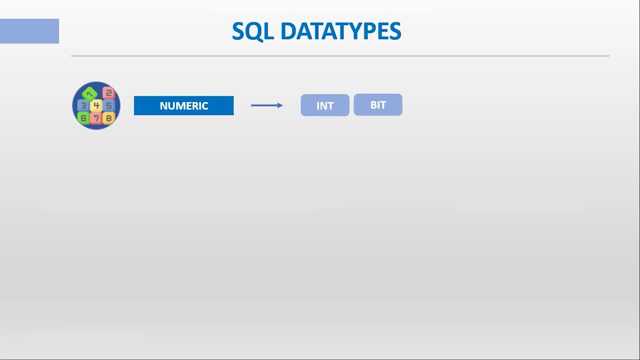 them as 1 byte. If a table has 9 or up to 16 bit columns, SQL stores them as 2 bytes, and so on. Float. Float stores the numbers having decimal values Depending upon the number of digits after the decimal point. SQL gives the size accordingly in its range. 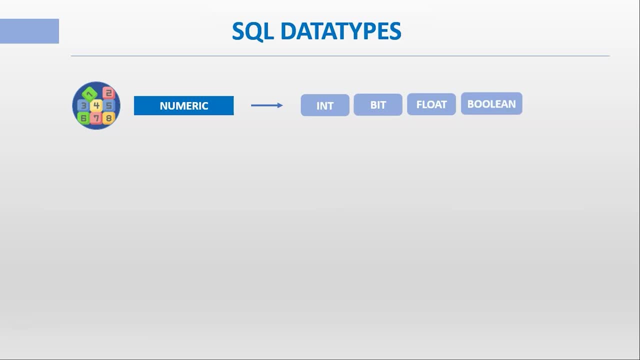 Boolean. It is used to specify Boolean values. that is true and false. 0 is considered as false and non-zero values are considered as true. String data type. String data types allows us to store fixed or variable character values. They are again further divided into various types. The first one is char. Char is a variable. 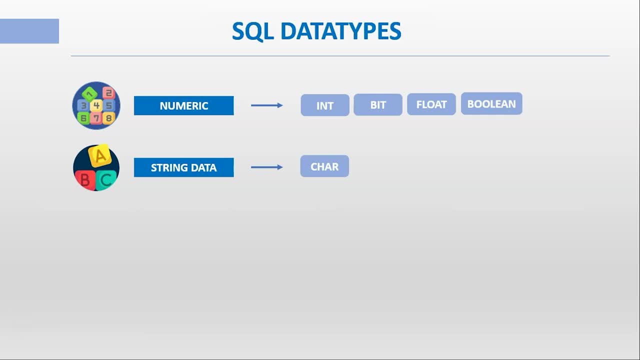 string. Char is used to specify a fixed length string that can contain numbers, letters and special characters. Its size can be 0 to 255 characters. VAR char. VAR char is similar to char, but it stores variable length strings, and size of VAR char is also more than the char data type, with a range of 0 to almost 60,000 characters. 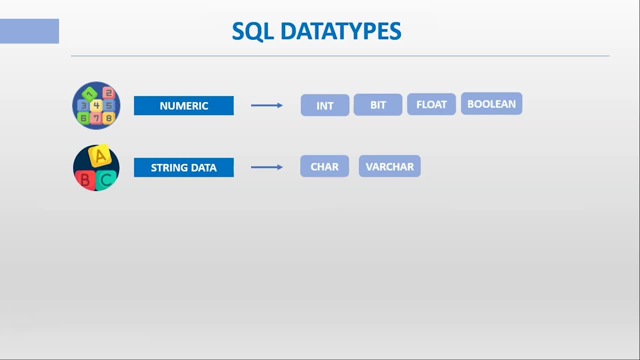 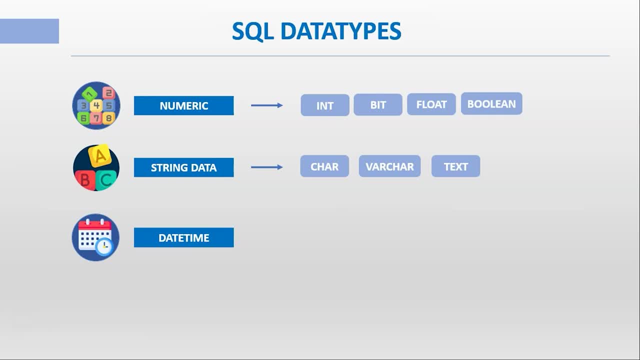 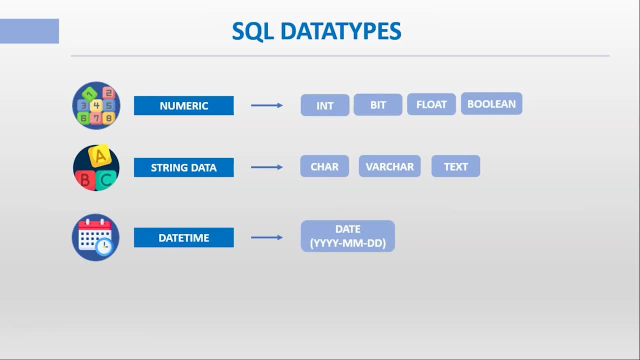 In this data type we can store only the value of date. Third one is DateTime. It is used to specify the combination of both date and time. The format is Year, month, date, hearts, minutes and seconds. We canaré store only the date value of due date. 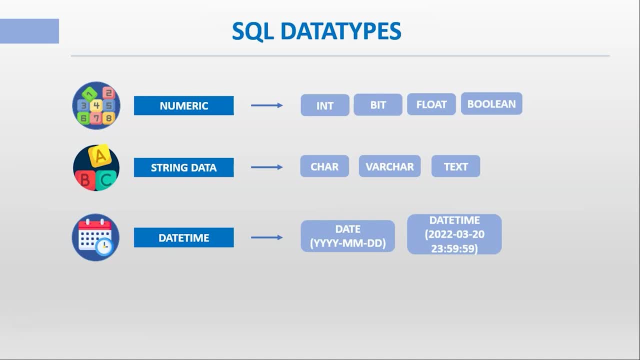 For instance, the example as 20, 22, 3- that is the month, 20 is the date, 23 hours, 59 is the minutes and 59 is the seconds timestamp. it is also similar to day daytime data type. the format specification is also the. 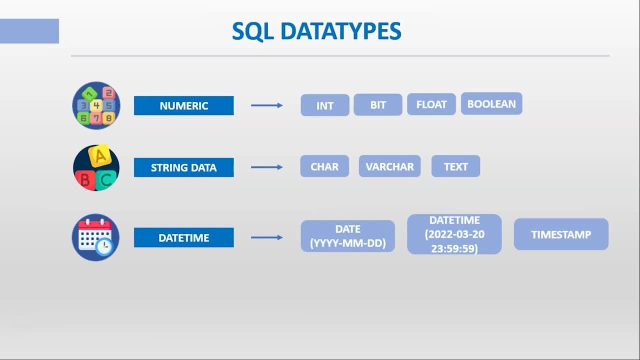 same as well. the only difference is it has less range of values to store. it is also used to convert current time into various time zones like utc, gmt, etc. we also have xml and json data types, which are not that significant and we do not use as frequently as other data types in sql. 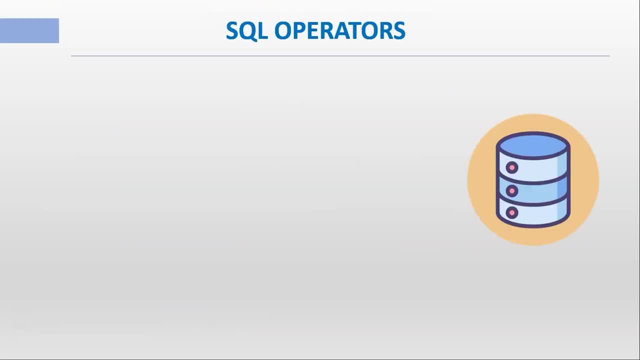 sql operators. sql operators are used to specify certain conditions in an sql statement. sql operators are broadly classified into five categories. the first one is arithmetic. arithmetic operators perform mathematical operation on numerical data on the sql tables. this operation performs addition, subtraction, multiplication and division operations on the numerical operands. the next one is logical. 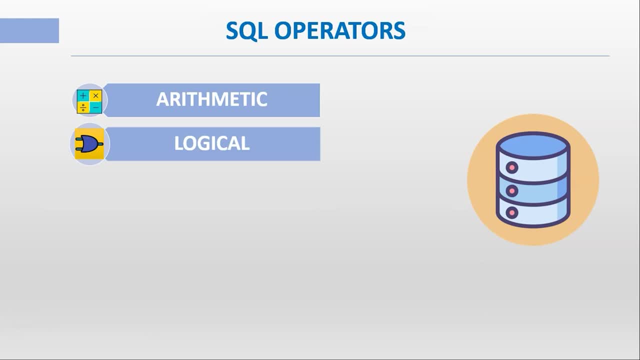 the logical operators in sql perform boolean operations, which gives two results, either true or false. these operators provide true value if both operands match the logical condition. some logical operators are and not, or between and out of the logical condition. comparison: the comparison operator is in sql. compares two different data in the sql tables. 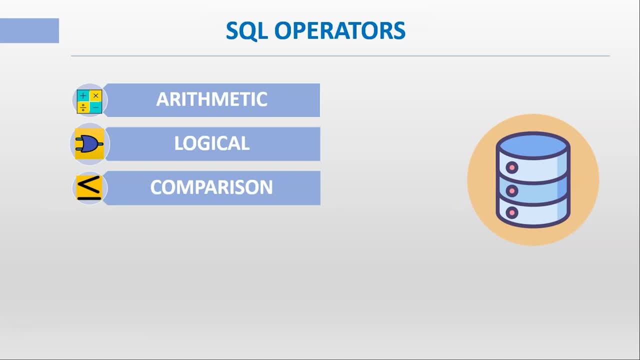 and checks whether they are same, greater or lesser. the sql comparison operator are used with a conditional clause where in the sql queries equal to is highly used a comparison operator in sql bitwise. bitwise operators perform bit manipulations between two expressions of the sql table. bitwise operators perform bit manipulations between two expressions of the sql table. 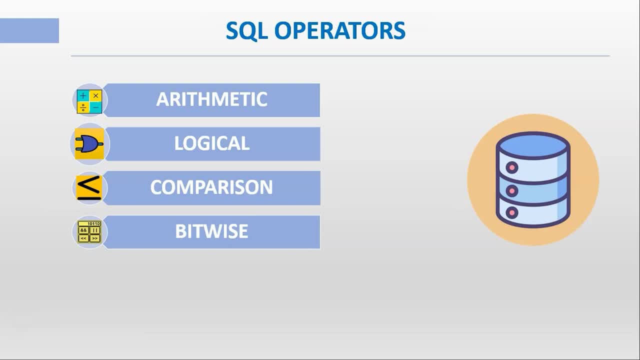 but twice. operators convert many integer data types to binary bits and perform and or or not operation of any integer data type category with host base. operators convert two integer values to binary bits and perform and or or not operation on each bit which finally gives the required result. 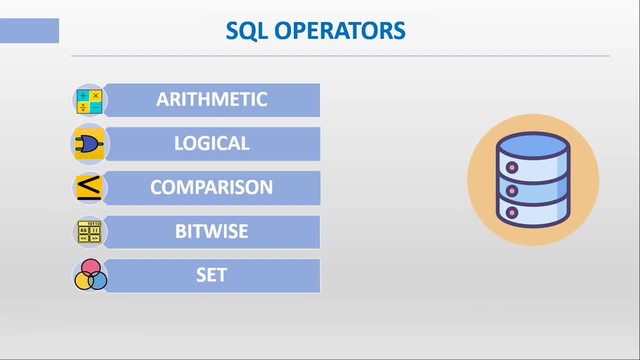 final one is set. the set operators in sql combine a similar type of data from two or more sql database tables. basically it merges the result which is extracted from two or more sql queries into a single SQL Union. Intersect and Minus operators are some of the examples of set operations. 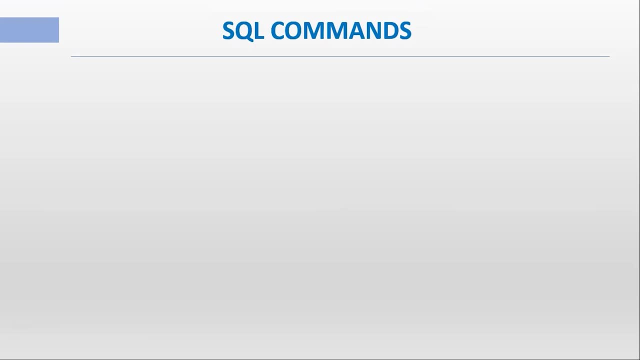 SQL Commands. We know that SQL commands are broadly classified into four types. The first one is Data Definition Language. DDL allows the user to define the table and make changes to its overall structure. Commands that are used in DDL are: It is used to create a new table. 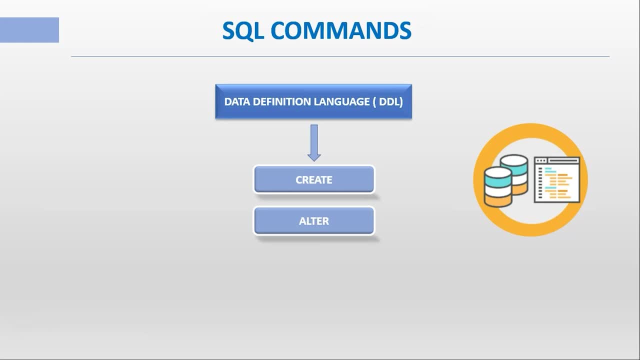 It is used to modify the existing table by adding new attributes. It is used to delete the whole table and the data stored in it. It is used to delete the rows in a table. Now that we have got the idea and understanding of various operators, data types and commands. 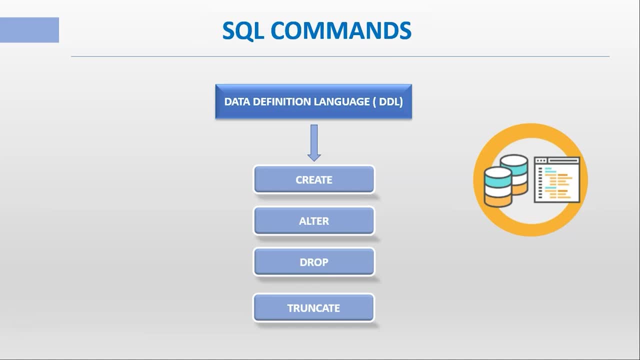 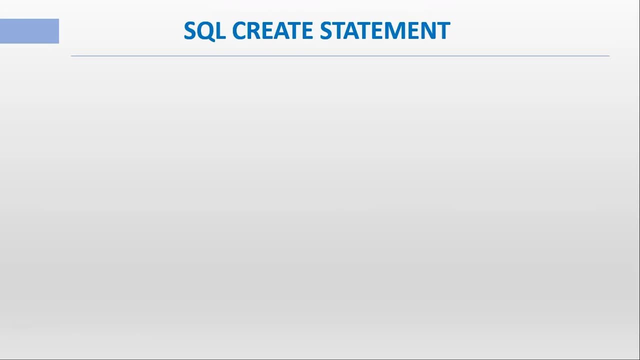 let us look at the syntax of all these commands. The first one is SQL CREATE statement, Perhaps one of the most important and used SQL statements, Because if you want to create a table, you have to first name the table and then specify the columns and the column data types. 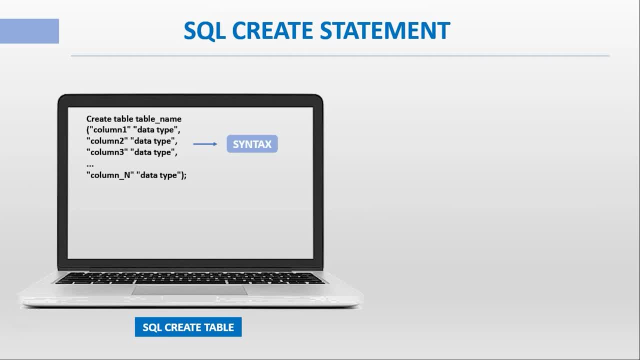 So let us look at the syntax of CREATE statements. The syntax is followed as CREATE table, which is the keyword that is used, followed by table name that you want to create, and within the parenthesis you have to mention the column, give space and add the data type. 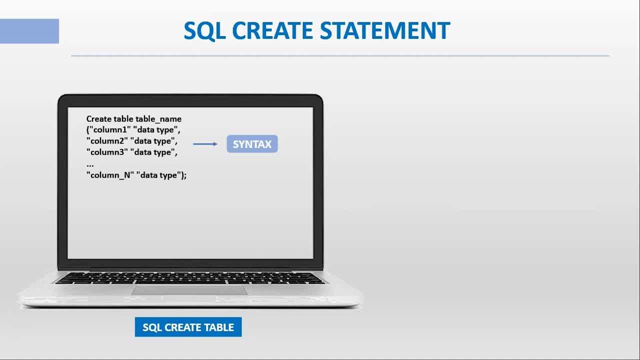 So in this way you can add n number of columns and mention the data types. But make sure, guys, you have to give the appropriate data type for the columns that you have taken, Because there might be an instance where you have given the column, such as age. 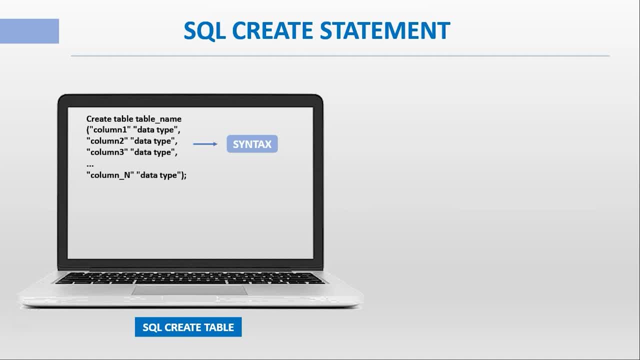 and you are mentioning data type as character char, which is basically a mismatch. The computer does not accept it Because generally age is basically a numerical value, but you are mentioning char. But it should ideally be int to store the data. 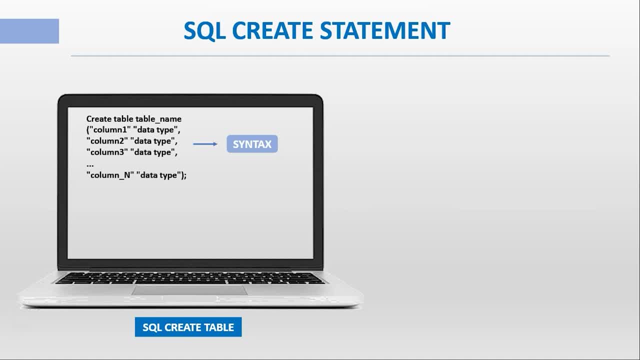 So just keep an eye on it when you are creating your tables. So let us now look at an example of CREATE statement. So I want to create a table named employee. For that I am writing as CREATE table employee And within the parenthesis I am mentioning employee ID as my first column. 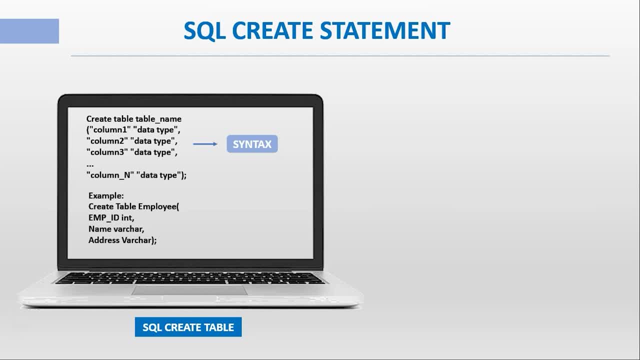 space int, which is the data type, And I am giving name varchar, address varchar, Close the parenthesis And put a semicolon, And if you execute this statement, this will be the following result: It will display the table with different columns. 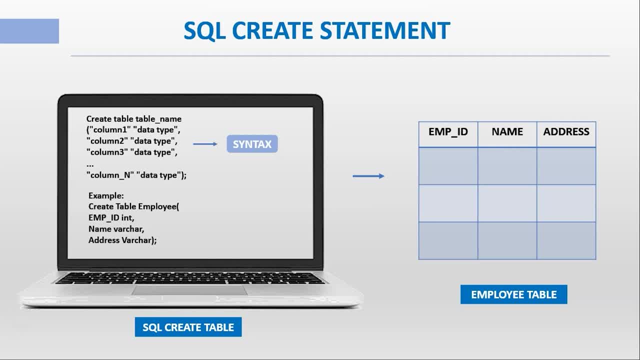 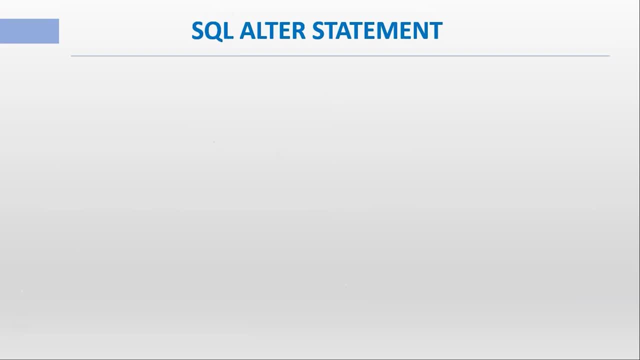 With the first column as employee ID, the second column as name and the third column as address. Easy right. The next one is SQL alter table. The SQL alter statement is basically used to add, modify or even delete certain columns from the existing table. 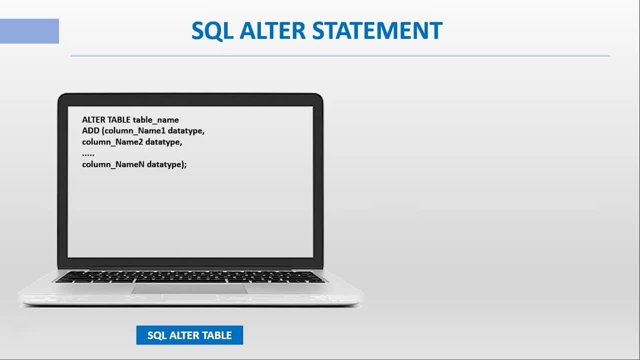 Let us look at the syntax of the SQL alter command. So the SQL alter command is alter, table, space, table name, that you have to mention add and within the parenthesis you have to mention the column and the data type. Similarly, you can add a number of data types as per your requirement. 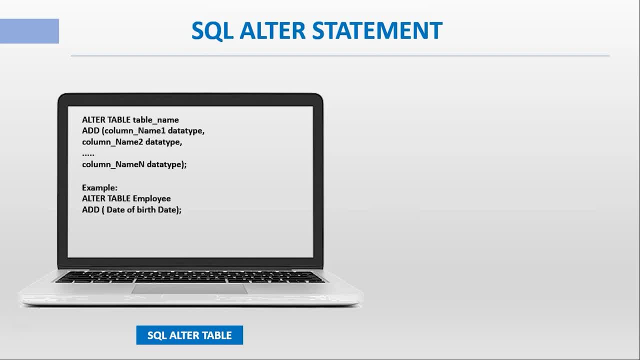 Let us now look at one of the examples. Now I wanted to add the date of birth of the employee in a new column. For that I am adding the date of birth. I will write as: alter table, employee add and within the parenthesis, date of birth. 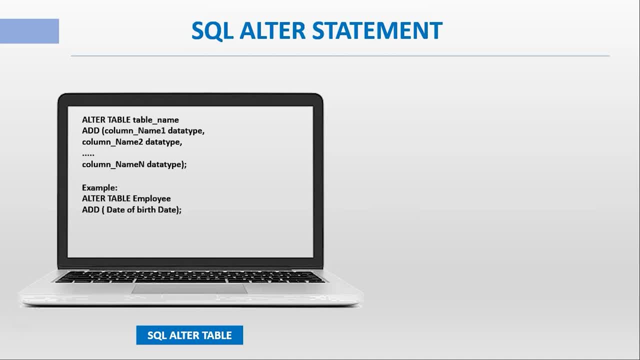 And I will mention the data type as well, which is the date, And if you execute this, it will show the result like this: It will add another column, date of birth- in the already existing table. Now, due to certain reasons, if you want to drop or delete the date of birth column, 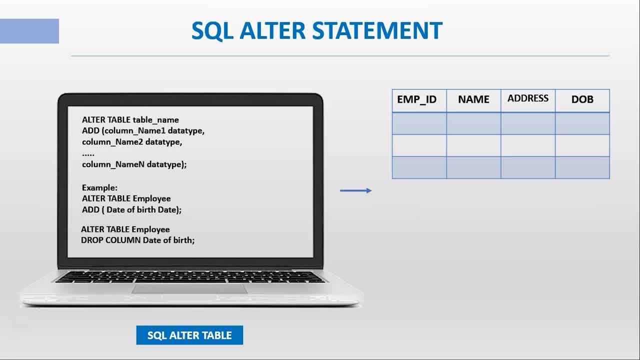 for that we have to write syntax as alter table. Give the employee table name, drop column, which is the keyword we use, and date of birth. So this will be the final output when you execute the query. It will completely drop the date of birth from the table. 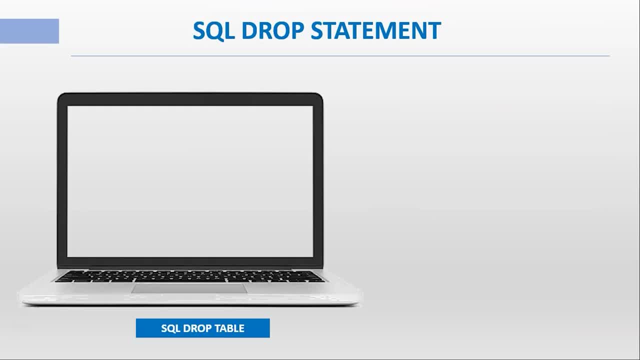 Next we will look at SQL drop statement. SQL drop statement basically removes all the data and changes the overall structure of the table by deleting the records in the table. So let us look at the syntax. The syntax followed is drop table, followed by the table name that we want to create. 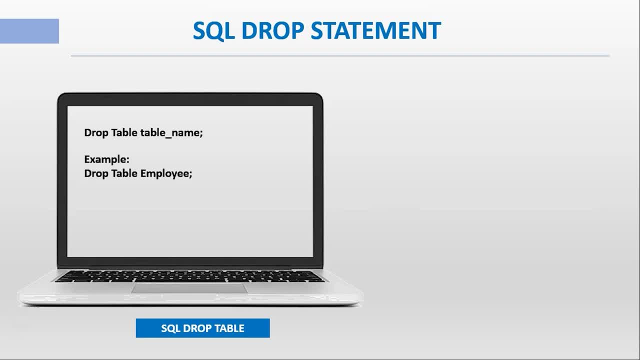 Let us look at one of the examples. The syntax followed is drop table employee And when I execute this, it will show an error stating that table employee does not exist, which means we have completely deleted all the records from the employee table SQL truncate statement. 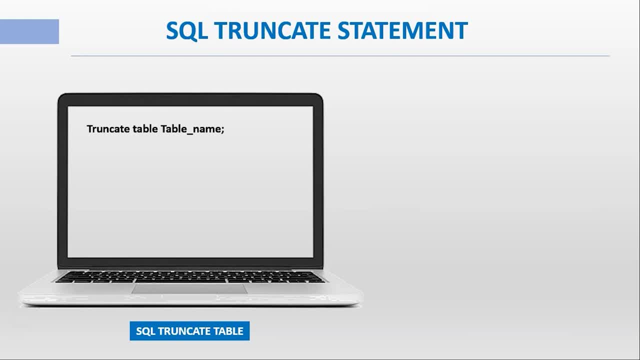 Let us look at the SQL truncate statement syntax. The syntax is truncate table, which is the keyword that is used, And we have to specify the table name. For example, if you want to truncate the values in employee table, we have to write truncate table- employee. 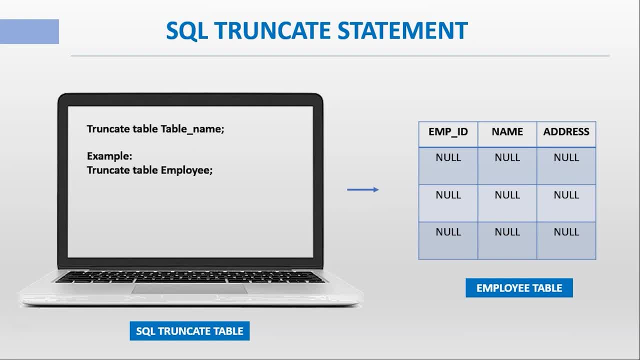 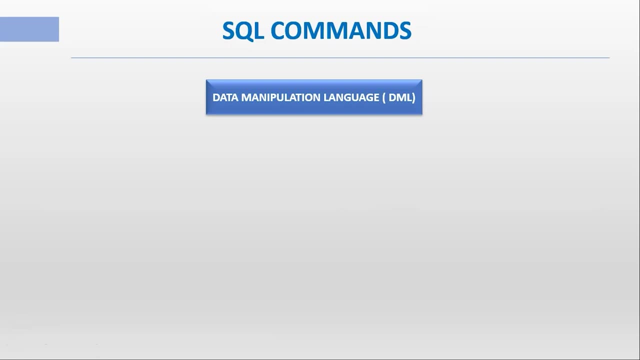 So this will be the output, where it shows null, That is, there are no values in the employee table, And you can further add values of your own choice. Let us now look at data manipulation language. Data manipulation language, or DML, is used to access and manipulate data tables. 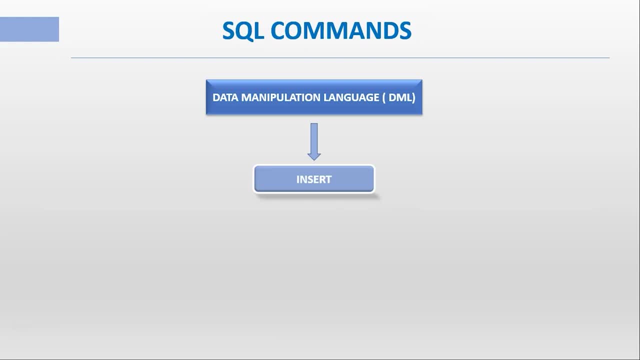 Commands that are used in DML are: insert: It is used to insert new values into the table. Select: It is used to extract data from the tables. Update: It is used to update values in the already existing table. Delete, Unlike the drop command. 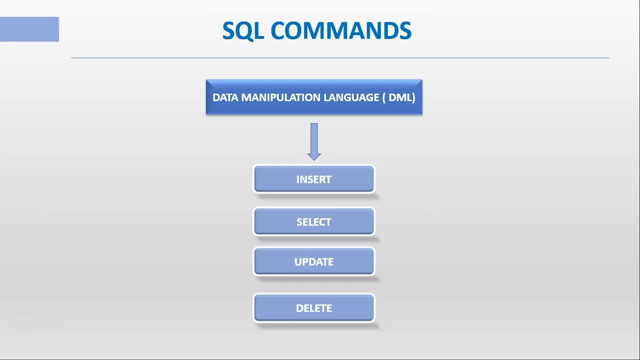 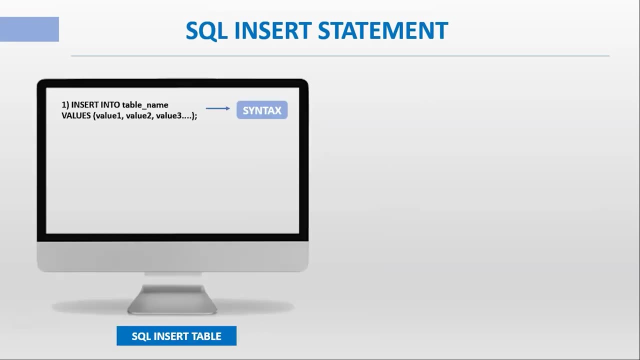 delete command is used to delete a specific row or all the rows in the table. Let us first look at the SQL insert statement. The syntax followed in SQL insert statement is insert, into which is the keyword that we use: Space table name that we have created. 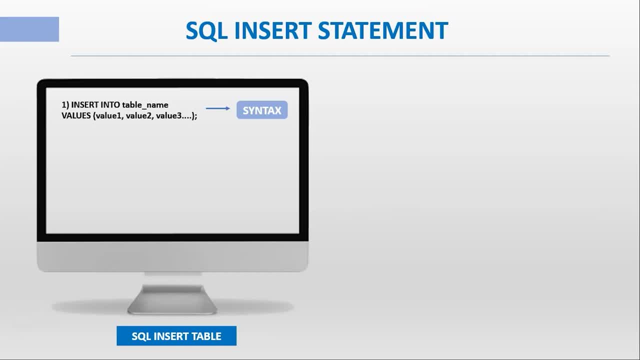 Values, and inside the parenthesis, you have to mention the values. There is also another method to insert the values, where we specify the column name as well as the values. Now, if you execute this, So, but before executing, we'll take an example. 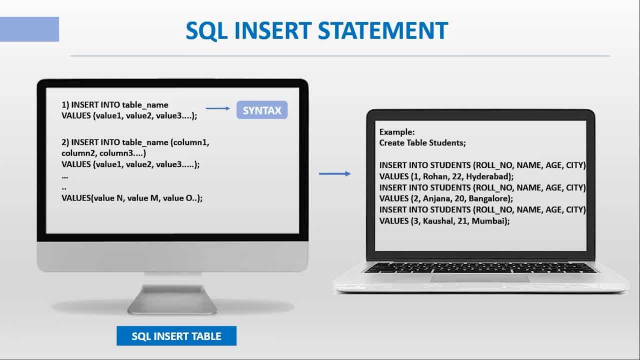 We are creating a table student and we are inserting values such as role number, name, age and city. So the role number is given as one, The name is given as Rohan, The age is given as 22. And the city is given as Hyderabad for the first row. 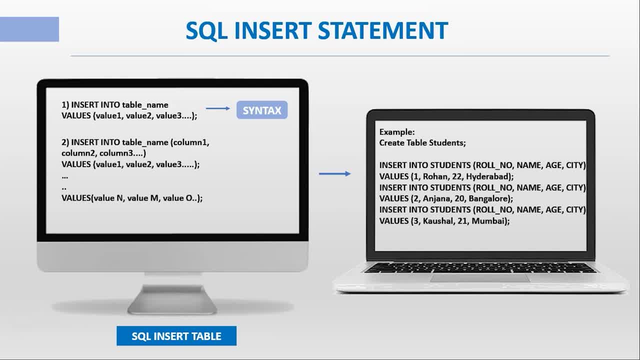 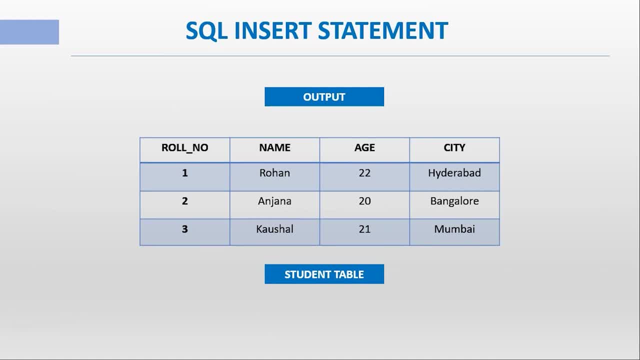 Similarly, we'll do the same for the next two rows as well, And if you execute this query, this will be the final output, where you'll have four different columns, Having the first column as role number, The next one having name, age, city. 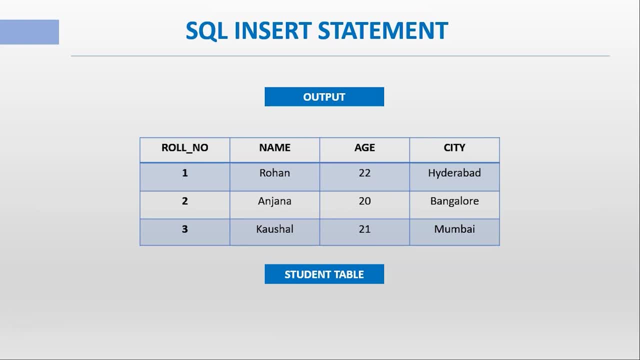 With the role numbers as one, Rohan, 22, Hyderabad, And the second row consists of the role number two, Anjana, age being 20 and the city Bangalore, And the third one is role number three. The name is Kaushal, age 21.. 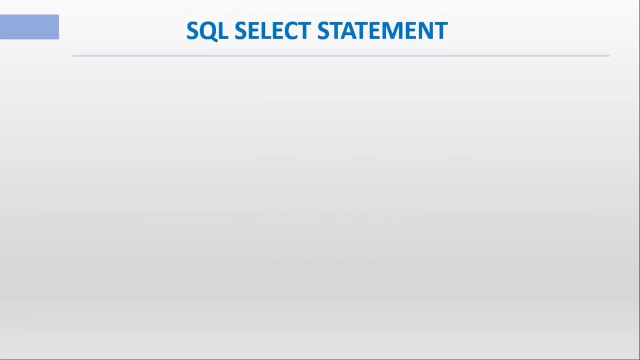 And the city is Mumbai. SQL SELECT statement. Let us now look at the syntax of SQL SELECT statement. The SQL is followed. The syntax is followed as: select column one, column two and n number of columns from the table name. And if you want to display all the names from the table, you have to use asterisk. 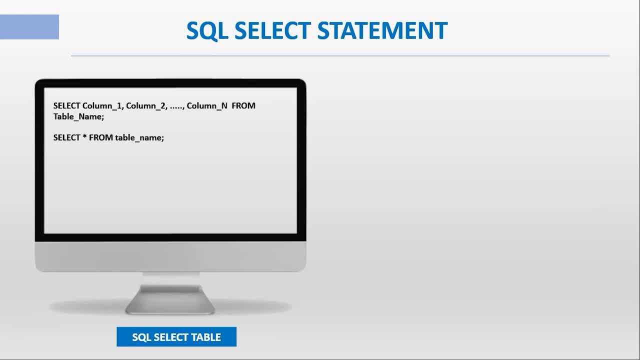 That is, select star from table name. Let us look at the example. So I want to display the role number, name, age from the student table. For that I'll write SELECT role number, name, age from the table. that is student. 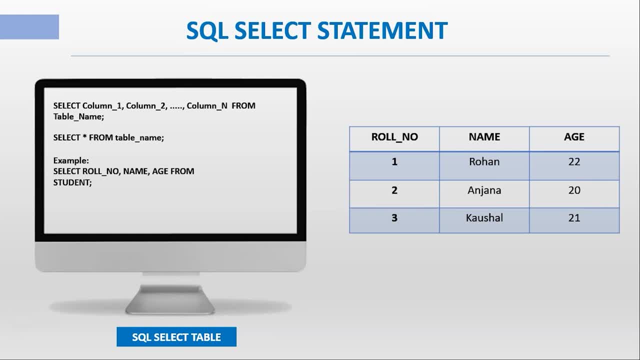 And if I execute this, it will only display role, number, name, age of the students And it will not display the city of the students. And if you want to display even the city To which they belong, We have to write SELECT star from student. 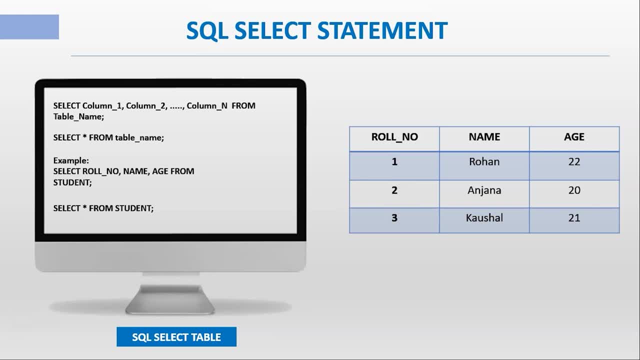 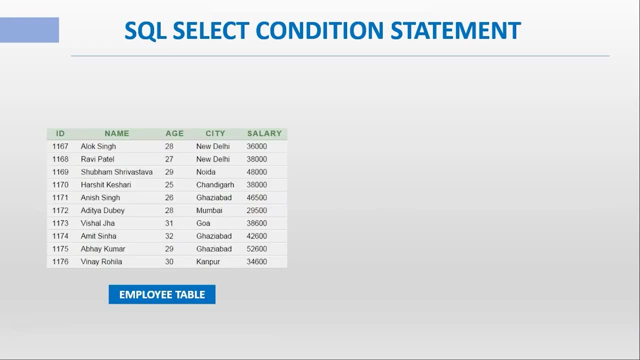 Then it will display even the city in the table. SQL SELECT condition statement. Consider the employee table with having ID name, age, city and salary And, if you want to specifically, you know, display the employee's name Who live in city New Delhi. 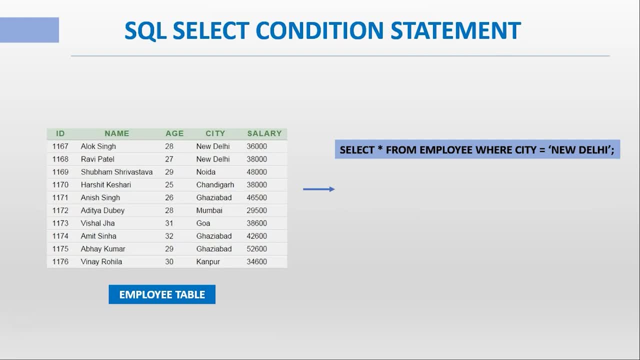 You have to write SELECT star from employee, where city is equals to New Delhi. Here we are applying a condition that is WHERE, Which is a SQL clause, And we are using an operator as well, which is equal to, And. if you execute this statement, 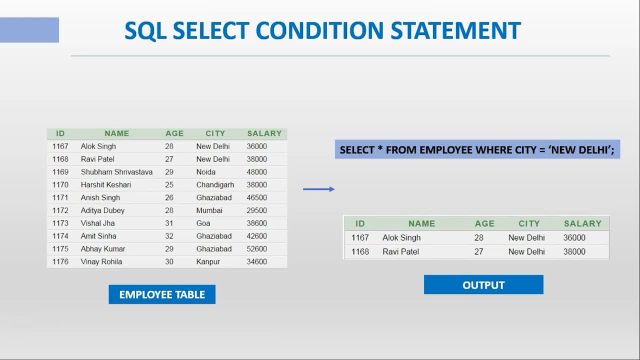 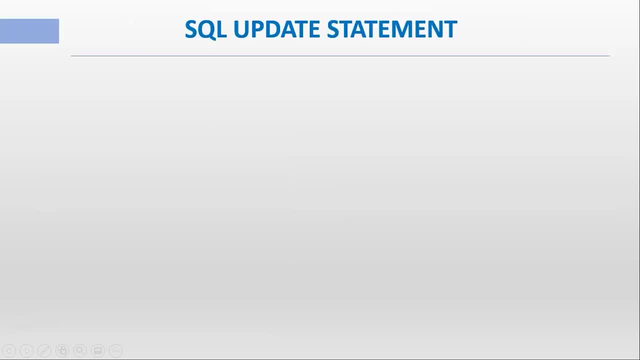 It will show this as output, Where you will find the ID of Alok Singh Ravi Patel, Who belong to the city New Delhi. SQL update statement. It is used to update Already existing values in the statement. For example, If you consider the syntax: 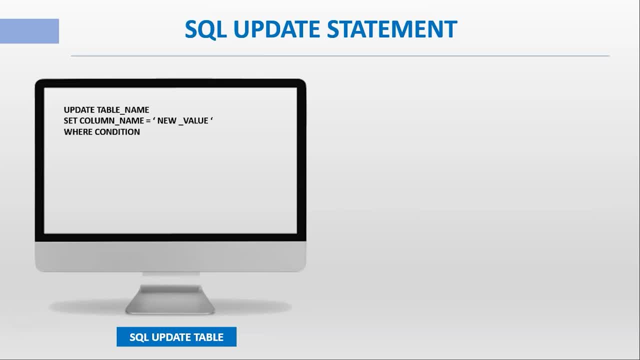 It is followed as Update space table name that you have created. Set column name equals to new value. That is the updated value that you want to keep into the new table. And you have to keep a condition as well. That is WHERE condition. 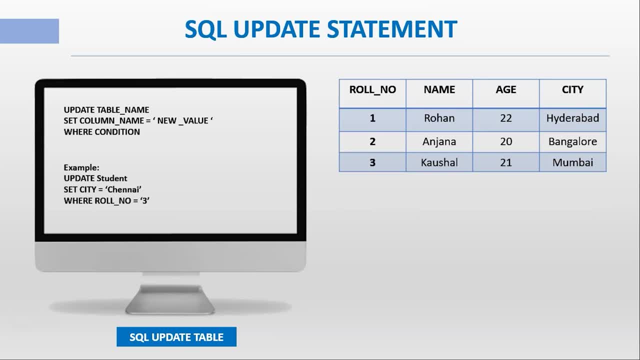 Let us look an example Now. if you want to update the student table And if I want to insert, If I want to change The city of the role number 3. That is Kaushal's city. I will write as: 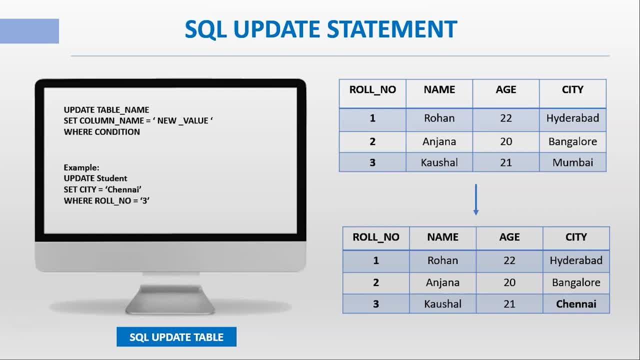 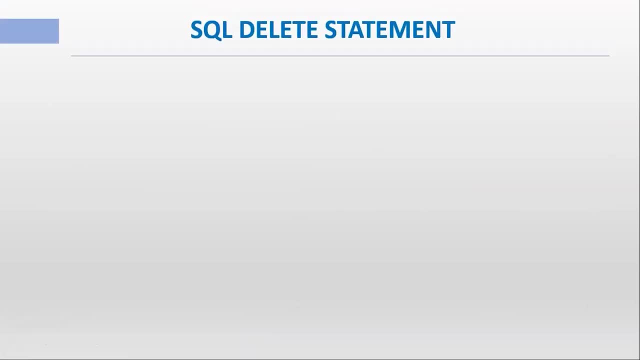 Update: student set city equals to Chennai, Where role number is equals to 3.. And when you execute this, It will show like this: So the city Which is Mumbai has been changed into Chennai. SQL delete statement. SQL delete statement Is used to delete a specific. 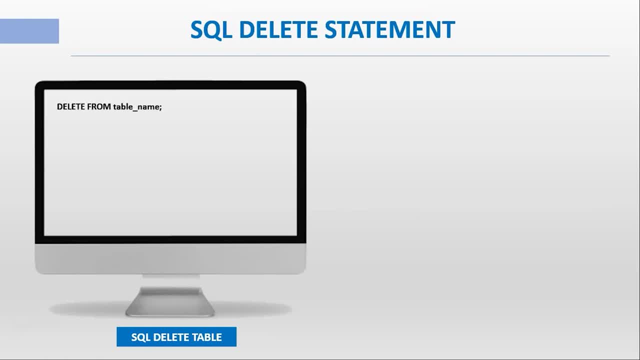 Or even all the rows from the table. The syntax is Delete from table name. For example, If you want to delete all the records from the student table, We will write it as Delete from student semicolon. So this will be the output. 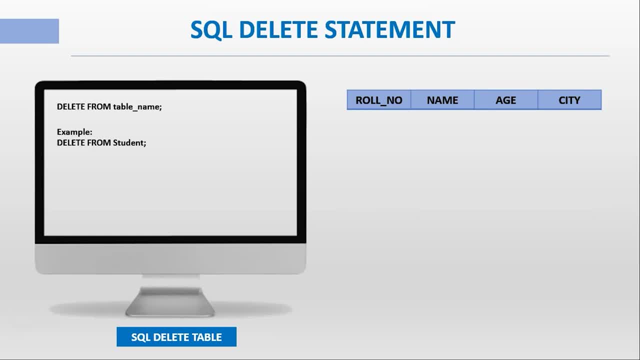 It will only display the column names And the data inside. it will be completely erased. And if you want to delete only a certain number of rows, We have to use query as Delete from student where role number is equals to 1.. And when you execute this query, 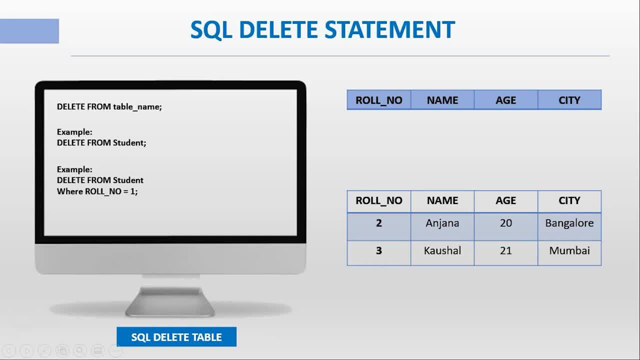 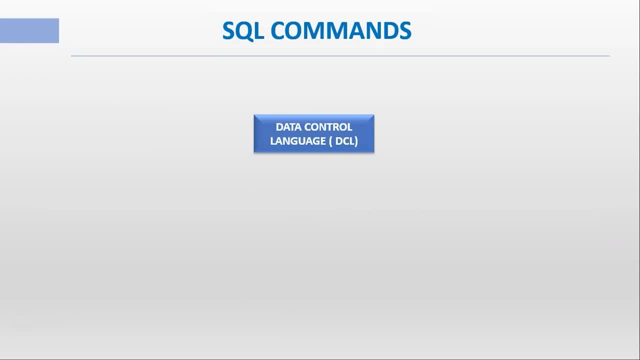 It will show like this: It will completely erase the records of the role number 1: student. And the final one is data control language, or DCL. DCL is responsible for maintaining the security Which gives control, access and permissions of the database. 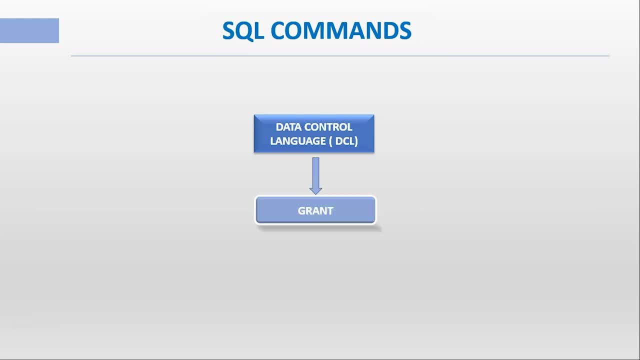 Commands that come under DCL are: Grant- It is used to grant the permission to user to access the database. Revoke- It is used to cancel or take back the permissions that were earlier granted. Let us now look at SQL grant statement. 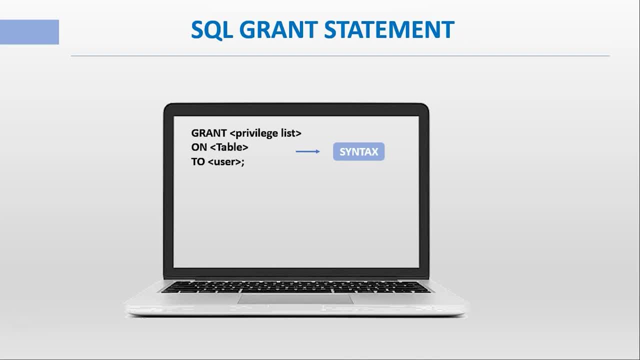 Sometimes user is restricted from creating or making any changes within the table, But with the help of grant statement We can give privilege to the user to create or modify the records in the table. Let us now look at the syntax of SQL grant statement. 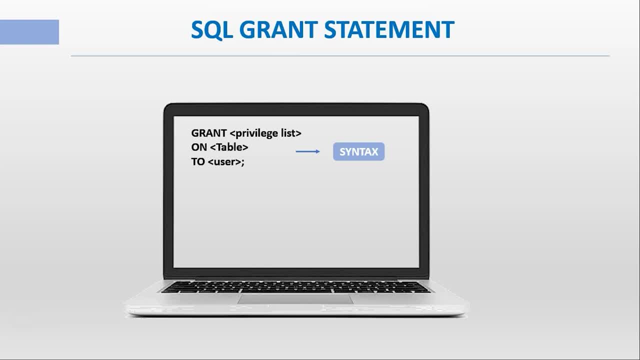 It is followed as Grant. It is provided in the default privilege list. That is basically the set of commands that you are giving access or permission to the user To perform certain operations On the table that you have created to user. We have to mention the username. 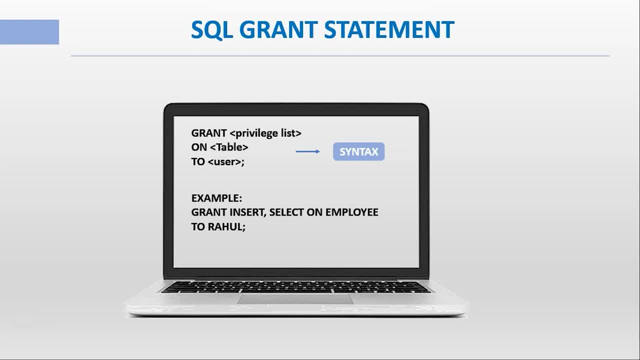 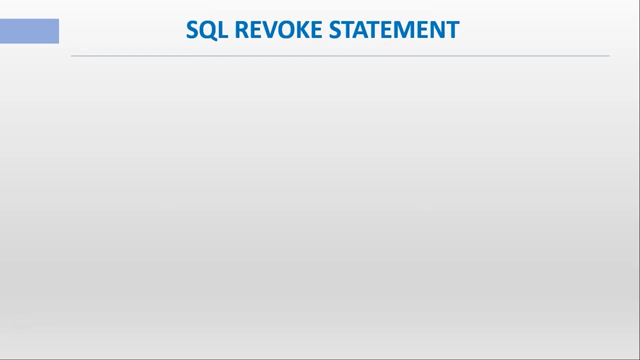 Example: Grant: Insert, Select on employee to Rahul. That means Rahul is able to access the employee table And can perform commands such as insert and select SQL revoke statement. SQL revoke statement. SQL revoke statement is basically the opposite of grant statement.